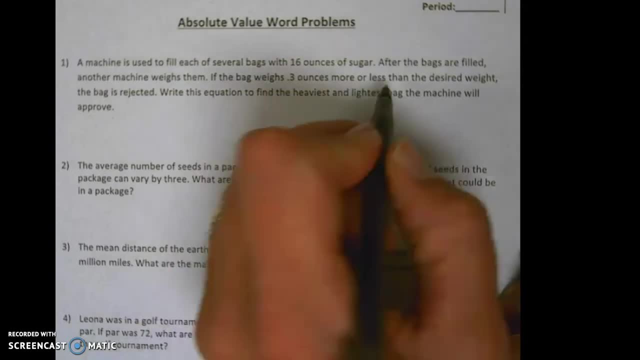 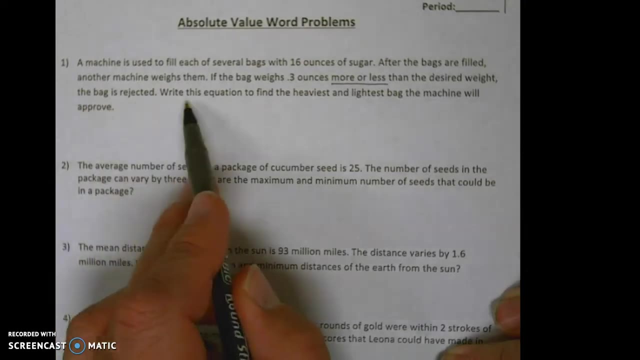 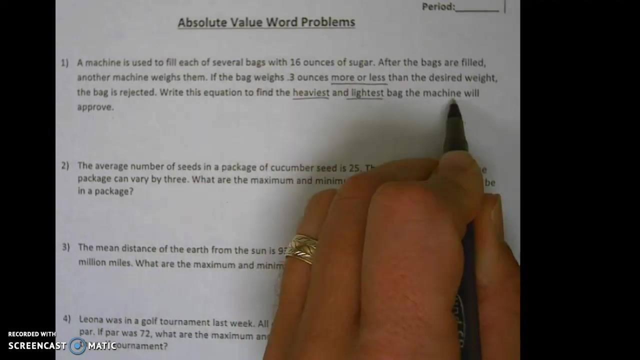 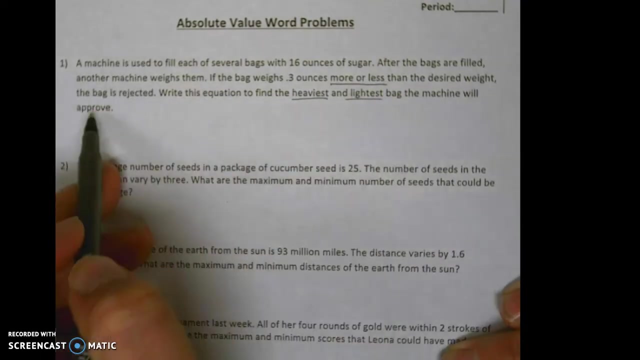 weighs point three ounces more or less than the desired weight, the bag is rejected. write this equation to find the heaviest and the lightest bag. the machine will approve okay. so, first of all, when we read this problem, how do we know that it's an absolute value word problem. well, 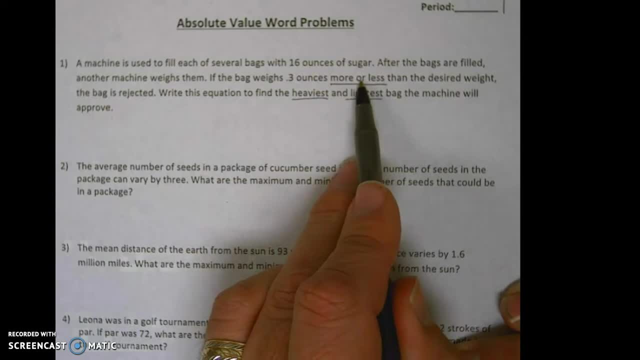 the key here is right here, more or less: okay, we can be above weight by point three ounces, or we can be below weight by point three ounces. so this is our margin of error, if you will. okay, so we need a variable. so what are we talking about here? 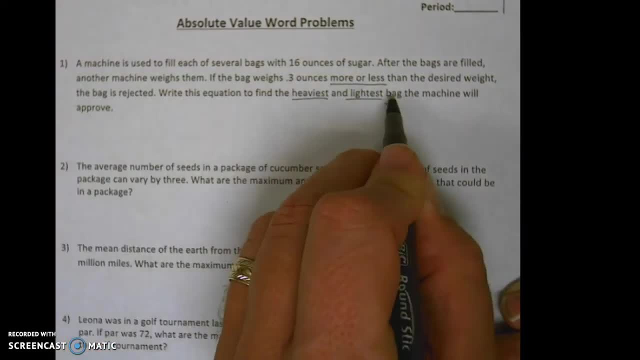 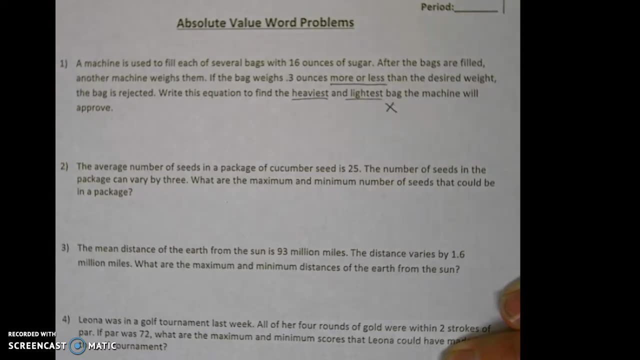 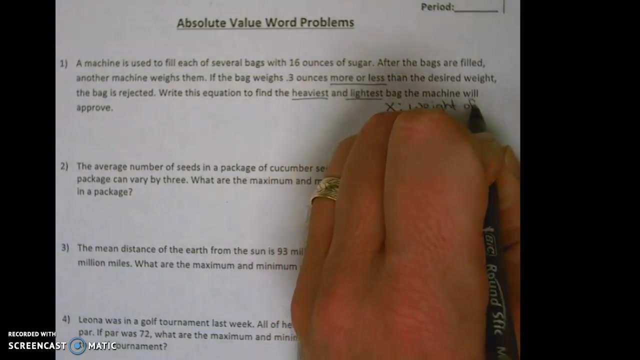 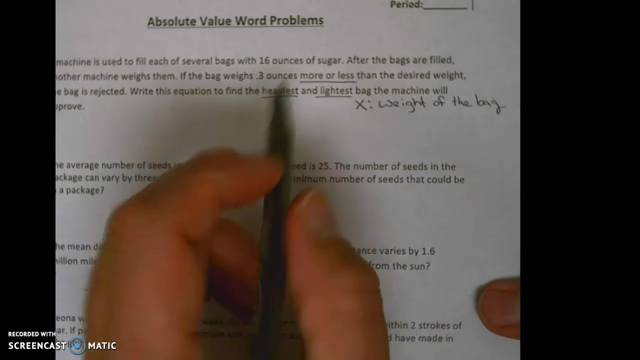 we're talking about the weight of the bag, the weight of the bag, so we're going to go ahead and use x, and it's going to represent the weight of the bag, okay, and so we're going to go ahead and fill it with 16 ounces of sugar. 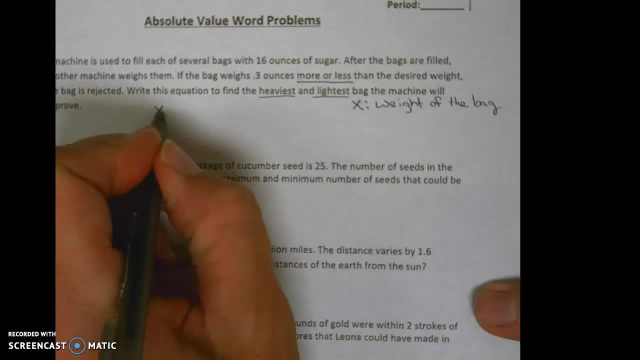 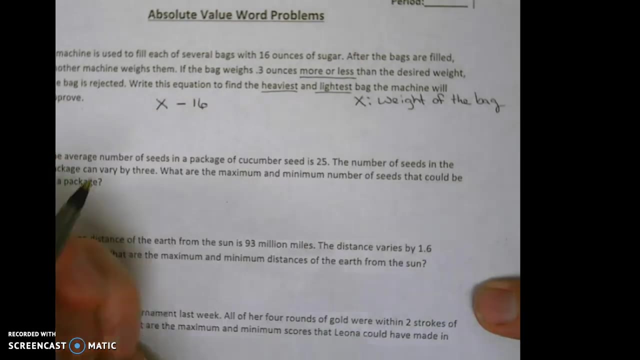 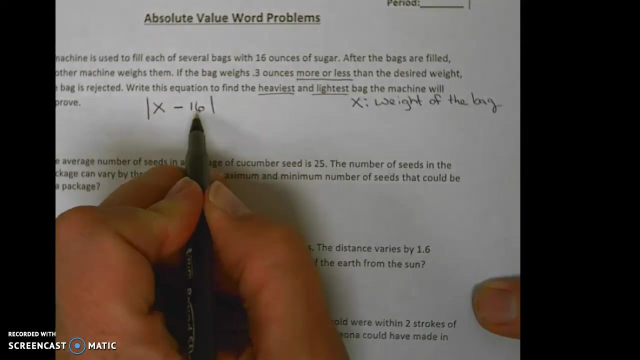 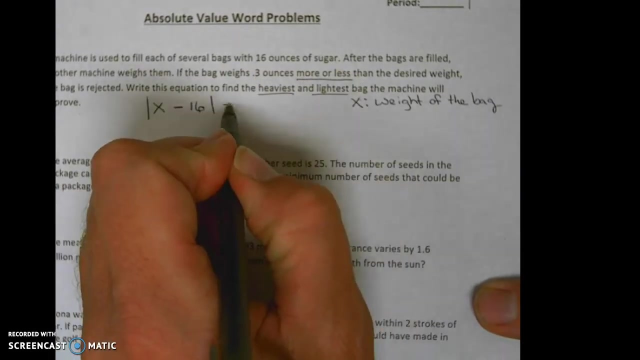 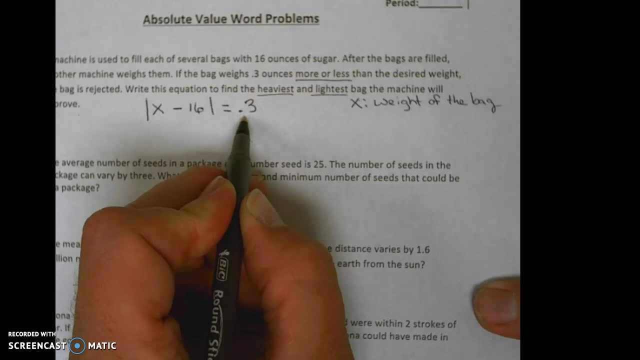 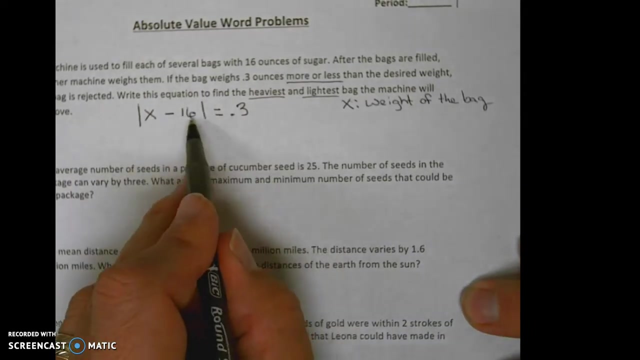 okay, so the weight of the bag, and we're going to take off the 16 ounces of sugar with absolute value around that, and the weight of the bag cannot be more or less than point three. so this is our varying amount above and below. now remember, this number here represents the amount of sugar, so we 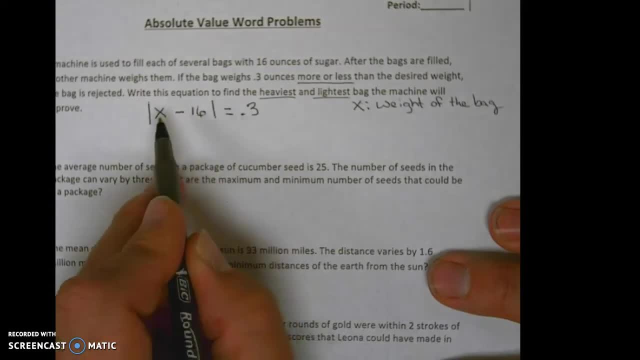 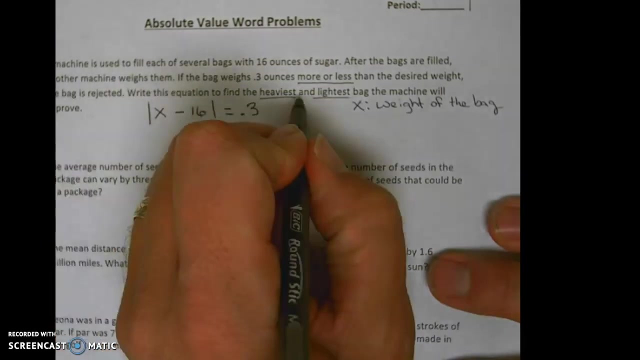 have to take that amount out of the weight of the bag, so that way we know how much the bag weighs. the bag can't be more than 0.3 or less than 0.3. so, solving this, let's go ahead and do the heaviest. 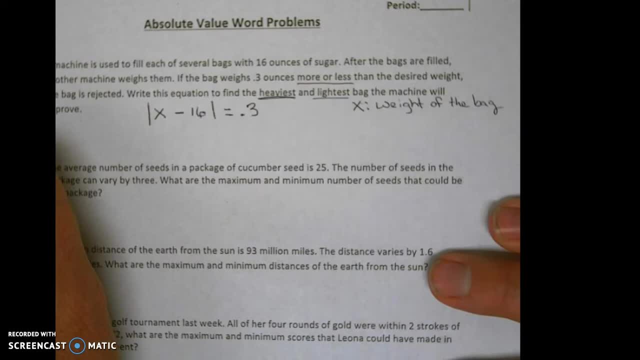 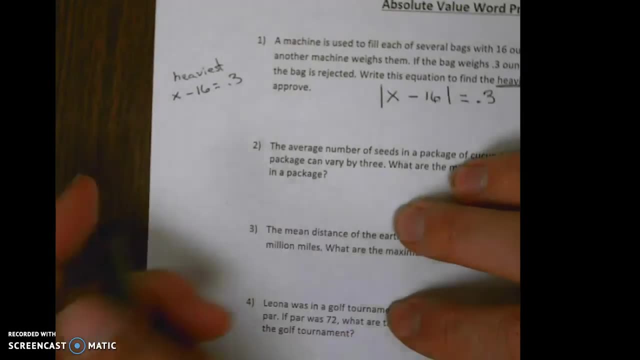 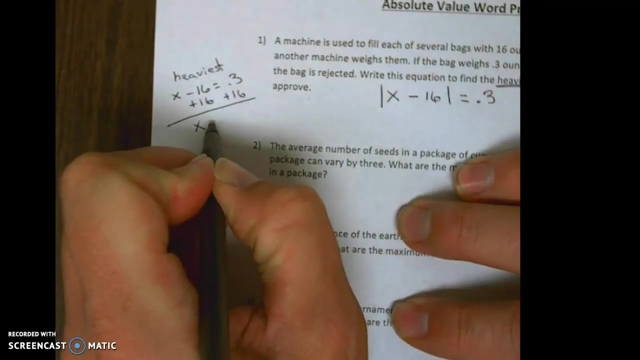 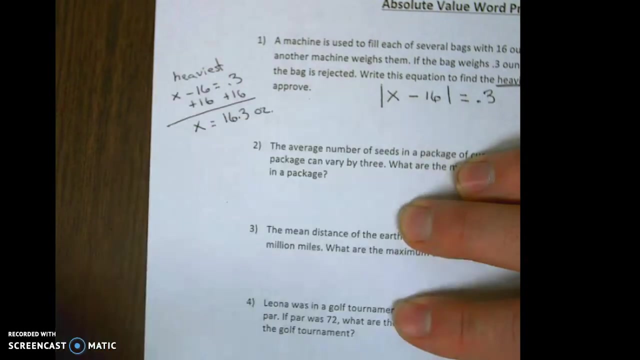 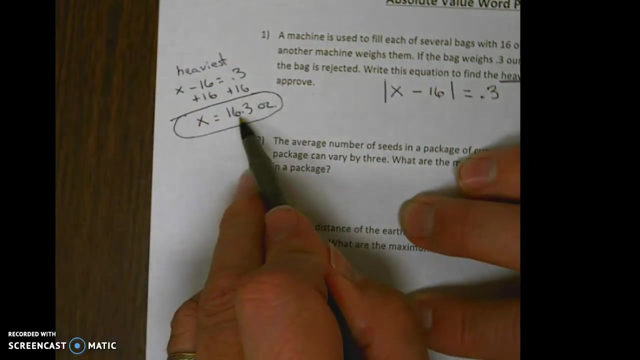 so that would just be basically: X minus 16 equals 0.3. so I'll do that over here on the side, adding 16 on both sides. so the weight of the bag can be 16.3 ounces. that's the heaviest the bag can be. notice: you have the sugar and then you. 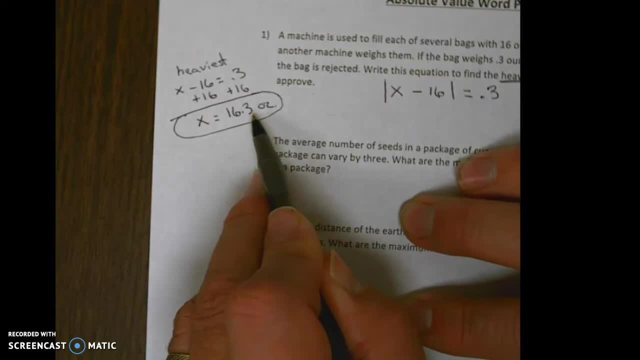 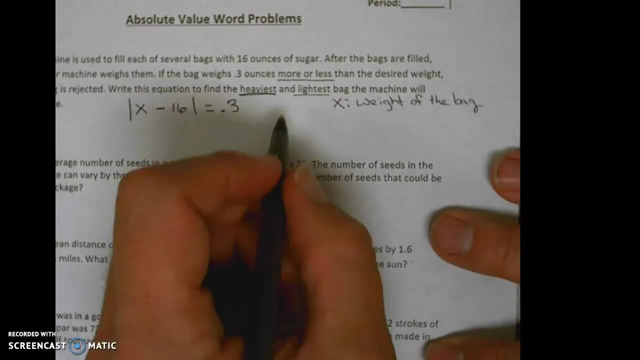 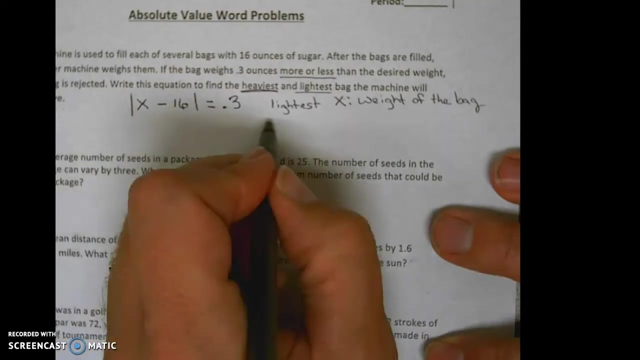 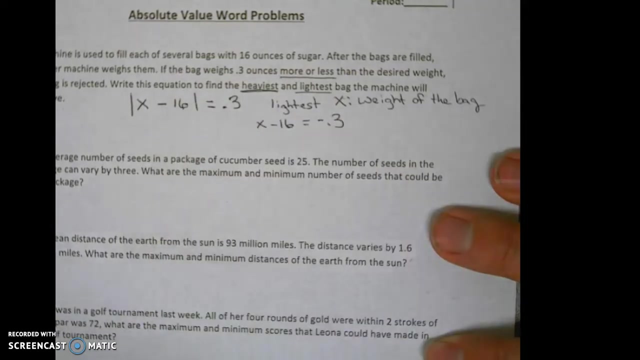 have your margin of error: 0.3. you can be above 5.3. okay, so now let's look at the lightest that the bag can be. so the lightest is going to be the other equation. follow along. remember, when solving an absolute value equation, you set one equation equal to. 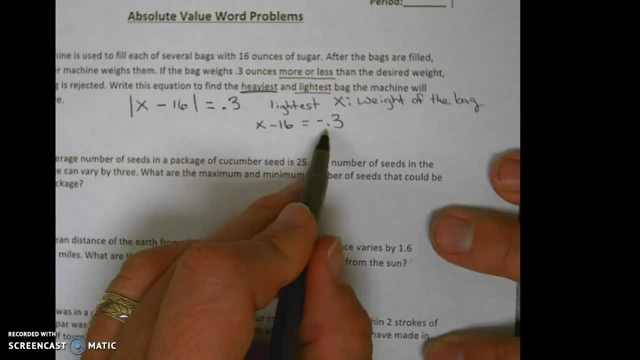 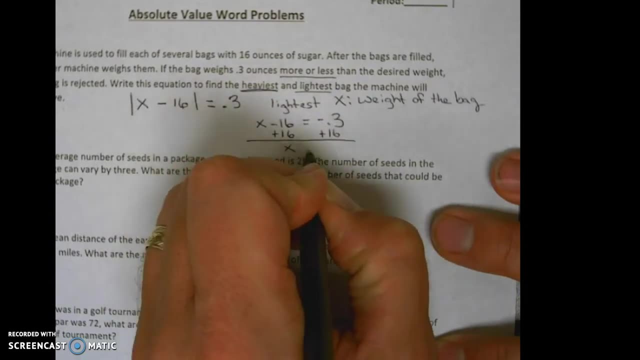 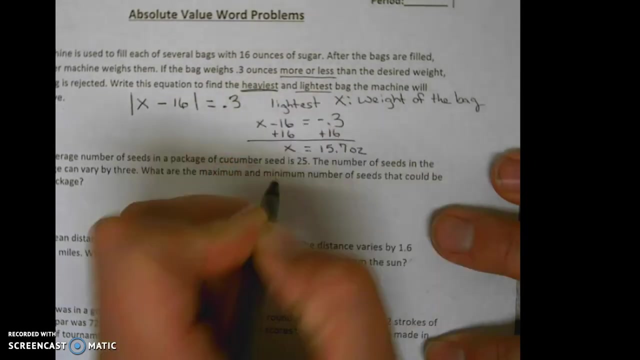 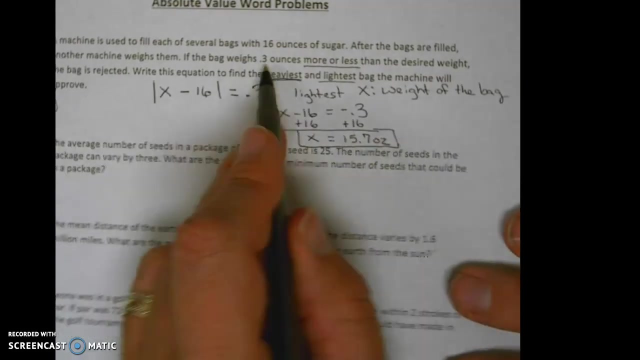 the positive and one equation equal to the negative. so solving this, one for X we'll get. X is equal to 15.7 ounces. that is our equation. it's the lightest the bag can be, so we can be 0.3 above or we can be 0.3 below. once we have added the sugar in. okay, let's take a look at number two. the average number of seeds in a package of cucumber seed is 25. the number of seeds in the package can vary by three. what are the maximum and minimum number of seeds that could be in a package? now you need to look for patterns. I have. 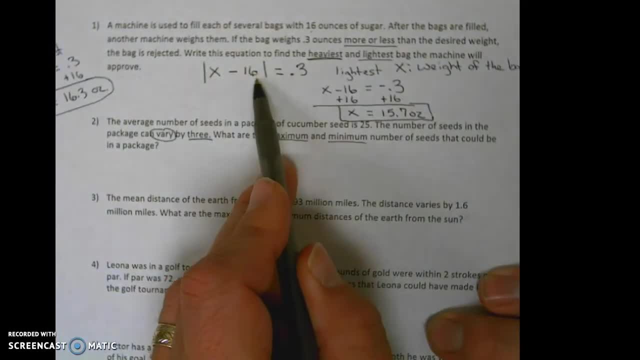 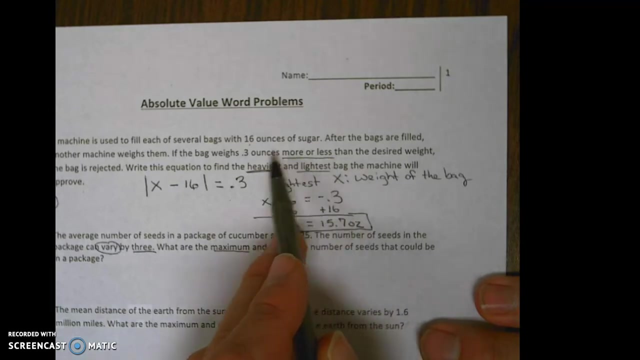 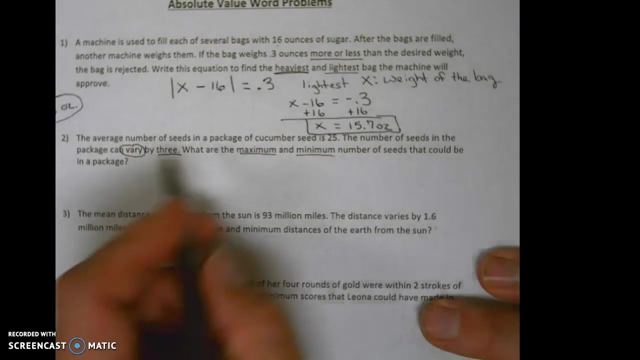 provided you an example on how to set this up and basically this is going to be your template for setting up the rest of these variables. so right away here, they didn't say very, they said more or less, more or less: point three ounces. here the variance is three. so obviously we're 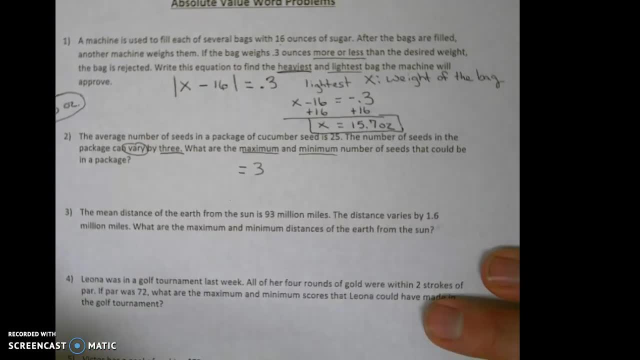 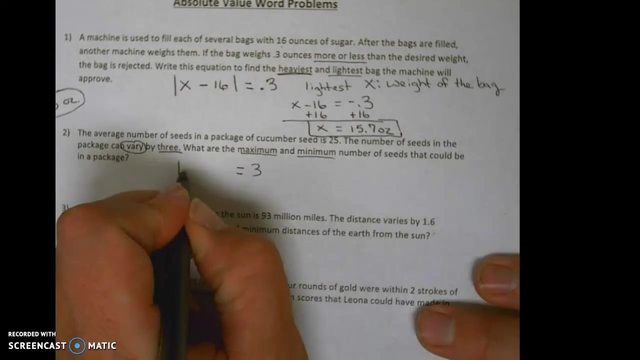 going to be setting this equal to three. we can be three above, which would be the maximum, or we could be three below, which would be the minimum, and then the the seeds is 25, so we're going to do the absolute value of X minus 25, and X is